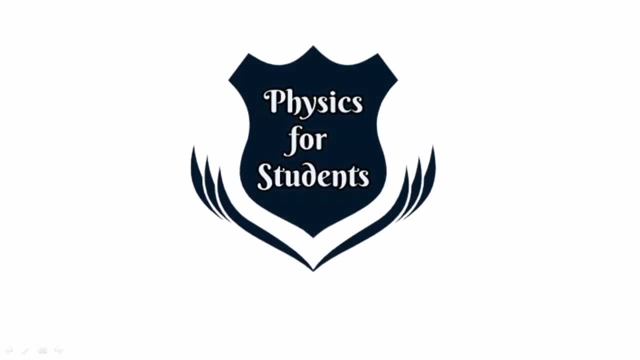 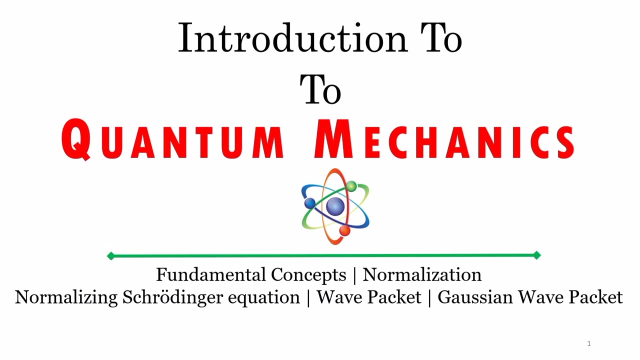 In this video, I am going to talk about some of the fundamental concepts of quantum mechanics. Among them, the first would be: what is normalization? Why do we need normalization? And some of the examples of normalization using Schrodinger's equation and Gaussian wave packet. 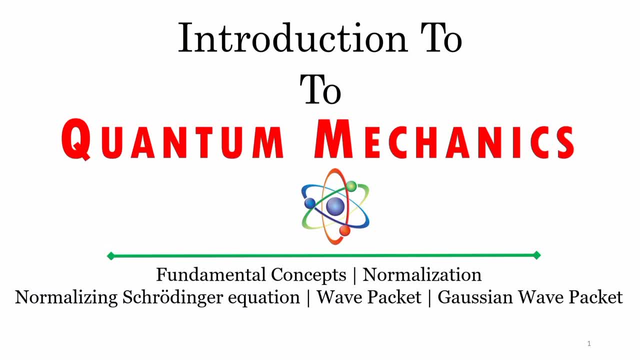 And definitely I would be explaining you what is a wave packet In this process. I would be explaining certain fundamental concepts of quantum mechanics And in this series of videos of quantum mechanics I would be sticking to those concepts, using mathematical equations and making it pretty simple, easy, so that you don't face any problems. 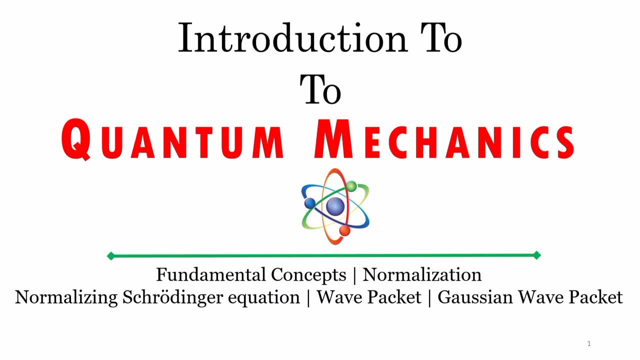 in further studying quantum mechanics in your further syllabus or studies. My name is Seanak and you are watching this video on my channel, Physics for Students. A warm welcome to this series of quantum mechanics. Now, before we start and go ahead into the topic details, first let us look into a quick recap. 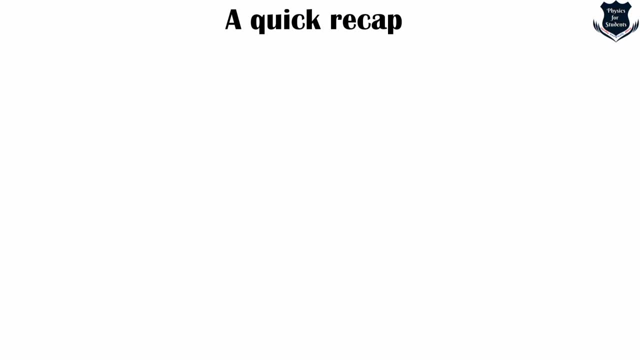 And I would request everyone to look into those recap concepts And if you have not gone through it, I would request you to go to my playlist In quantum mechanics, where I have few videos speaking on those, because these are very central before going ahead in the further complex and other concepts of quantum mechanics. 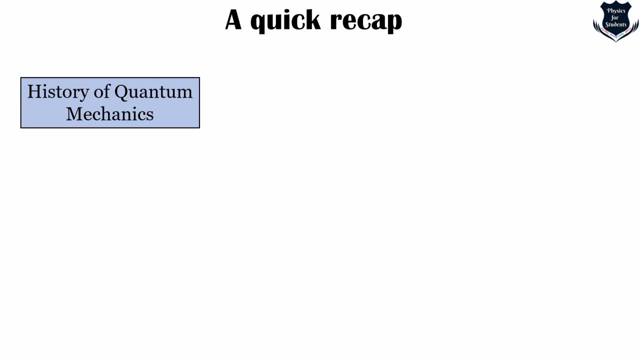 So first is that I have dealt a little bit about what is called the history of quantum mechanics, where I have spoken about how it evolved, who are the contributors, and also the Solvay conference, which is the pioneer moment of developing the history of quantum mechanics. 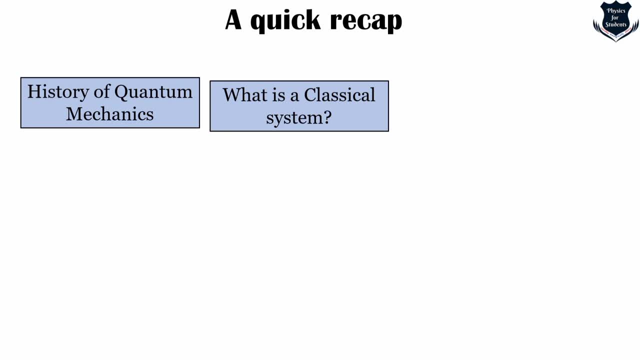 I have also explained what is a classic, And I have also explained what is a classical system, because there is a fundamental difference between a classical system and a quantum system. So it is very, very important for you to understand what is a classical system and what is a quantum system and what is the difference between those two. 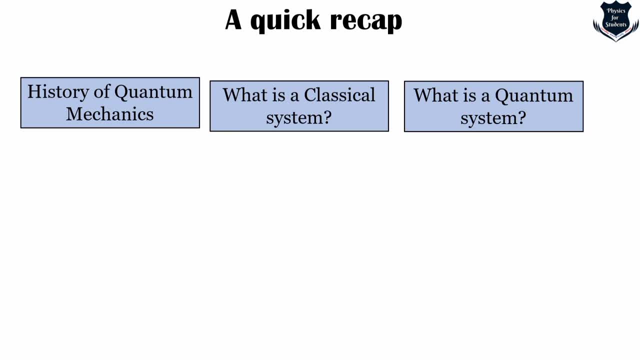 Because generally what happens for students? I have seen those who jump into quantum mechanics. they directly start with the probability wave function description without knowing what are the limitations of a classical system and why do we need a quantum system. Then I will explain what is a classical system and what is a classical system. 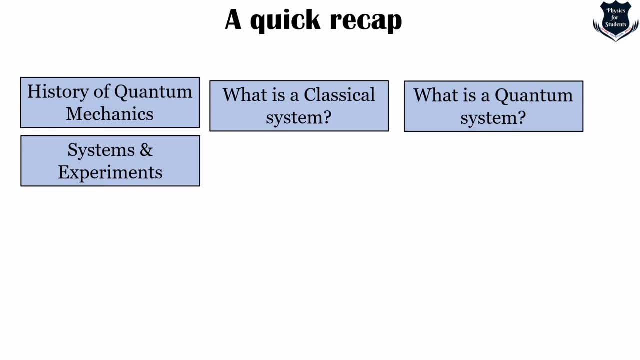 Then I would request you to look into what are the systems and experiments. In these videos I have explained more about how a system behaves and how the experimental outcome of a particular- I would say a classical phenomena yields to something totally different, which bypasses our general common sense. 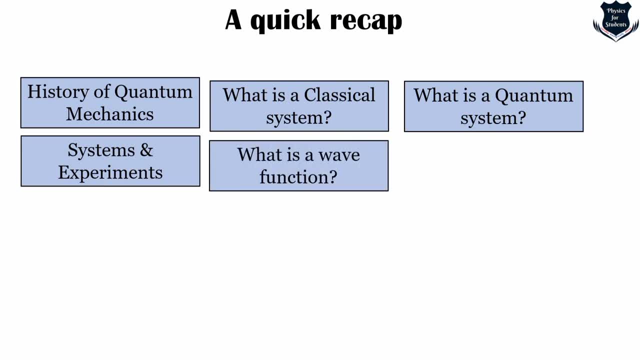 And that is the need and that is the bizarre world of quantum mechanics. I would also request you to have a quick look on what is a wave function, because this is central And I have dealt it in the other videos. Also the probability density, because the probability density actually gives us the exact or maybe a probable location in how to find out a particular subatomic particle and electron. 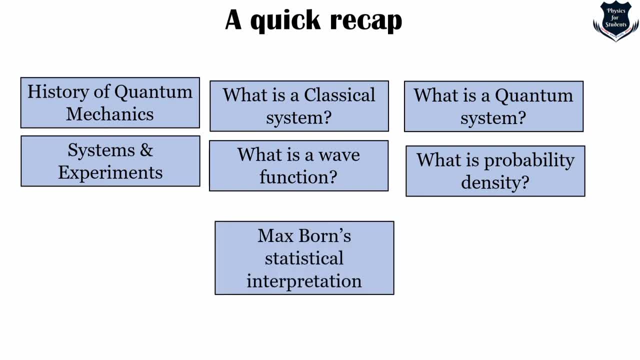 And finally, what is the Max-Wong statistical interpretation? that is, squaring the probability density, thereby finding out where could possibly the electron or the subatomic particle can be found. So history, The classical system versus quantum system, how the experiments yield different results. what is a wave function? what is a probability density and Max-Wong statistical interpretation? these are central. 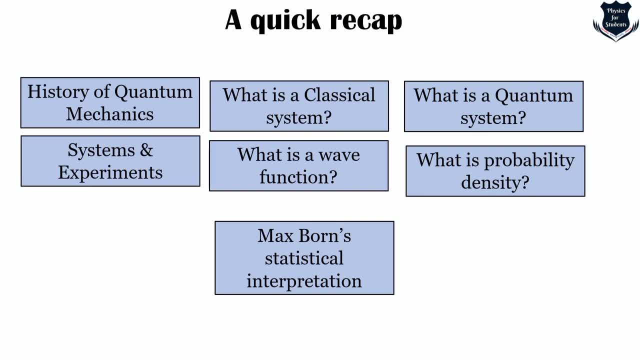 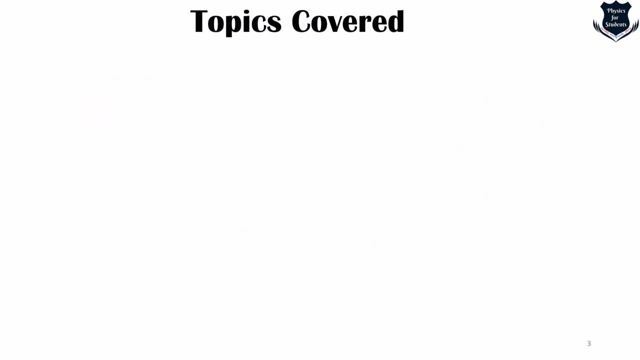 I am sure that you know all those things. In case that you don't know, I would request you to go to my playlist and have a quick look on those. I have explained it pretty simple, Okay. so what are the topics that we are covering today? 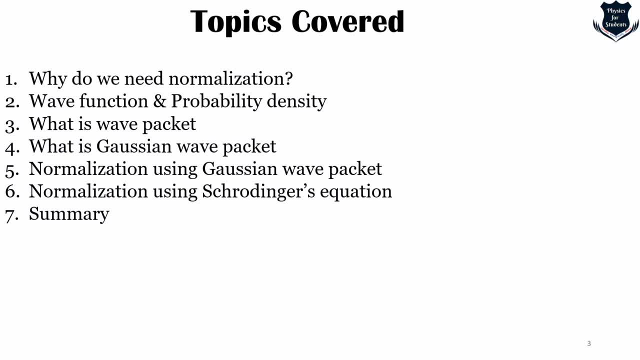 First we need to understand the need for normalization. Then we need to understand wave function And probability density. what is a wave packet? what is a Gaussian wave packet? what is normalization using a Gaussian wave packet? because Gauss's wave packet is very important. 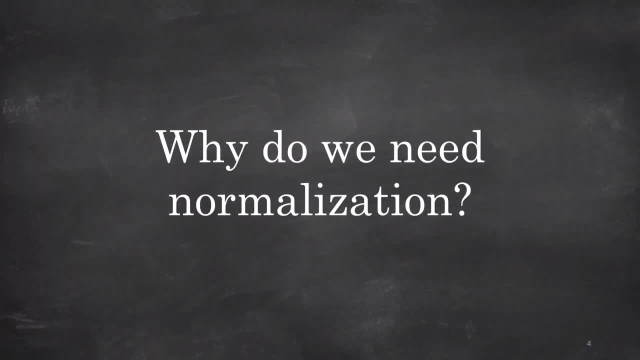 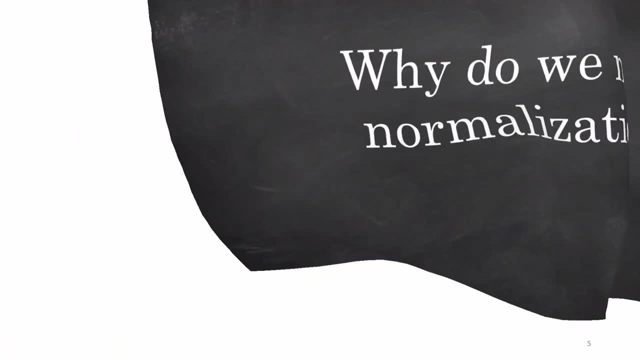 Normalization using Schrodinger's equation and the summary. Okay, so first, when we are talking of normalization, first we need to understand why do we need a normalization? Okay, so first I would like to explain what is a wave function quickly. 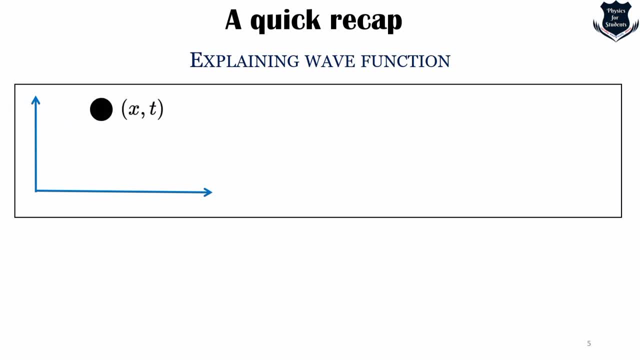 Okay, Here we have two particles, say for example this black one which is right on your screen. It has got a position and momentum which can be defined as x and t, And for example, if we get Cartesian coordinate two comma four, then we can probably understand what the particle is. 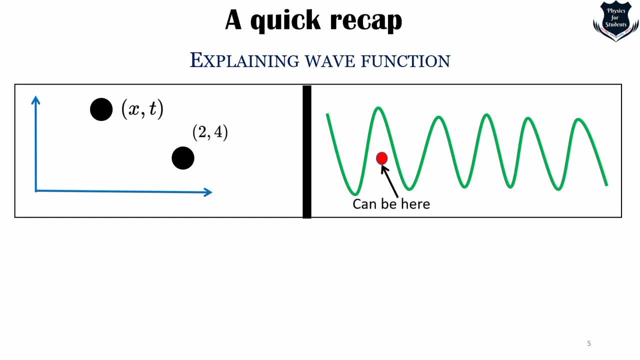 But on the right hand side, this wiggling green wave actually gives us a problem. The problem is that the electron can be here, It can be here, It can be here. So in a quantum system, in a quantum wheel, We really cannot find out a position or a momentum or anything that can directly locate the particle. 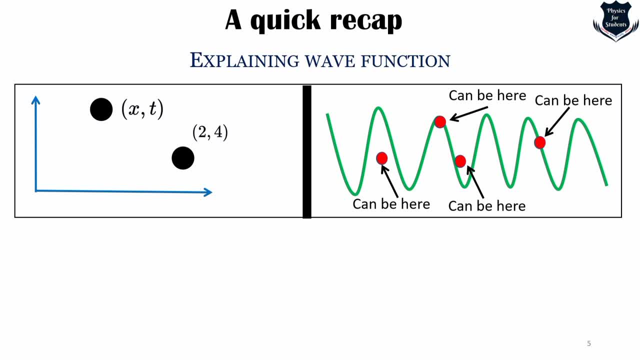 So it can be anywhere. So that is why I have given those red dots. That means it can be anywhere. Now. so the probability of the wave function in order to find a specific electron is denoted by this psi, this Greek letter psi. 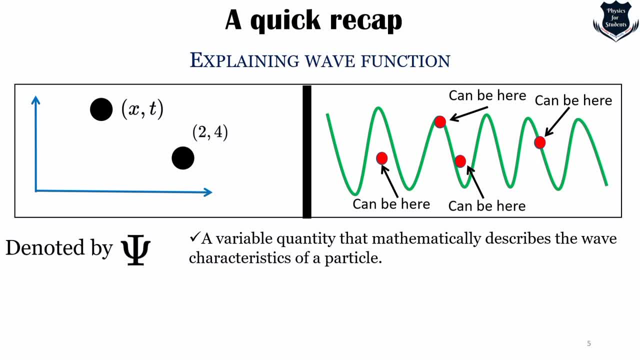 So what does this psi denote? It is a variable quantity that mathematically describes the wave characteristics of a particle. That means the probable location of that electron or a subatomic particle is denoted by the Greek letter psi. So the value of the wave function depends of a particle at a given point of space, and time is basically dependent on the likelihood of the particles being there at the time. 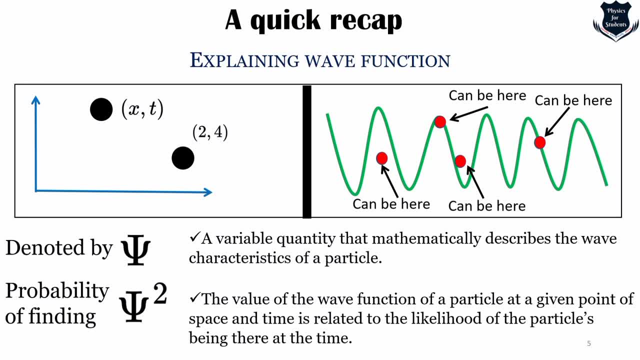 So that is what is called the probability of finding, is the squaring of the value of psi. That means where the electron is located, we really, really don't know And we can only find out. So first, the psi denotes a variable quantity that mathematically describes the wave characteristics, and the value of the wave function of a particle is related by squaring this psi. 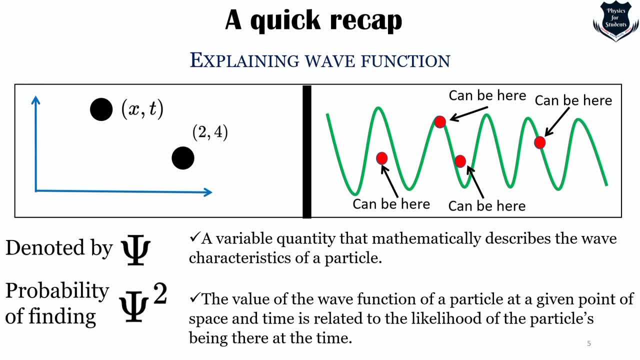 Now you see that the problem from classical mechanics to quantum mechanics, is unable to find out a specific location. That is predictability, And this is the reason that we need to do normalization. So first we understood what is a wave. Now, coming back to Max Bounce, 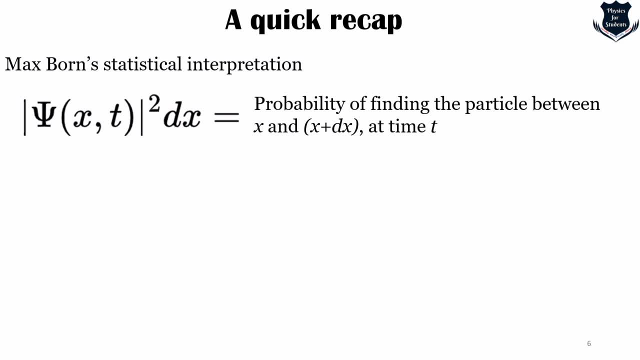 So in this statistical interpretation, you see, I have basically squared that which gives the probability density, So the probability of finding the particle between x plus dx and time t. So if I take this kind of a probability density where the x part is being squared, then I get a wave like this: 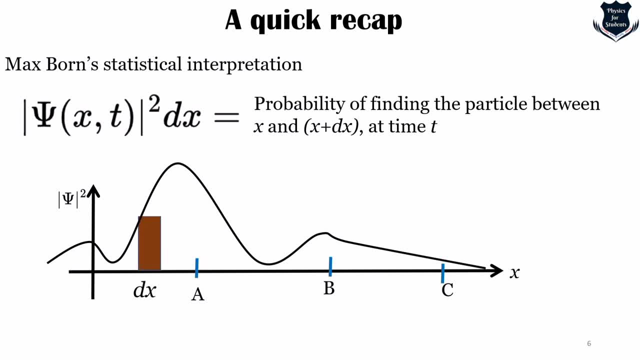 And then I mark points like a, b, c And the probability of finding the particle is this gray, you know rectangle part And this is where I can find the particle. So I can get a probability of finding the particle around a rather than b and c. 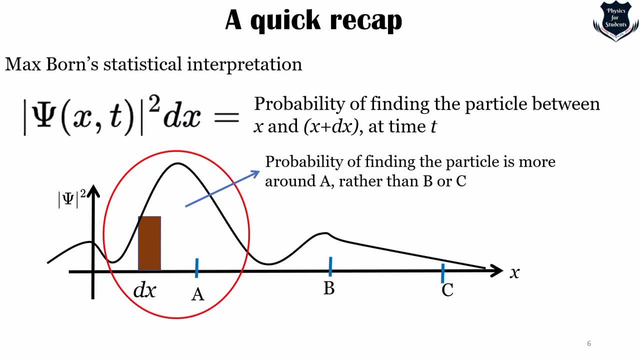 So the b and c part is excluded And my mathematical calculations, or our mathematical calculation, tells that the probability of finding the particle is around here Now, because it is a probability, because we are unable to predict a specific location. that is why we need normalization. 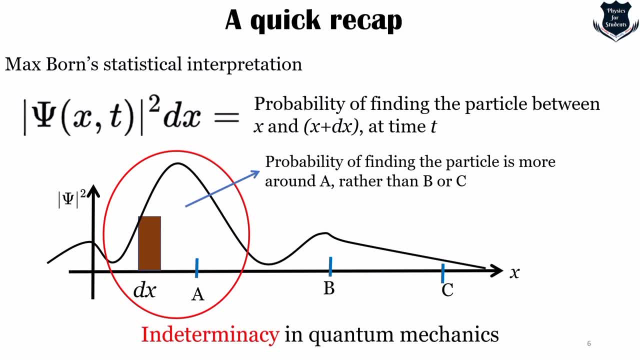 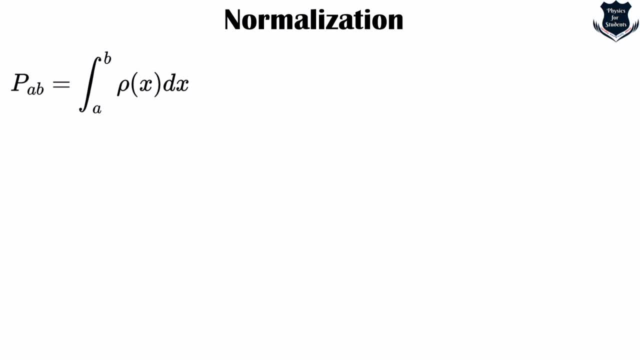 Because that is why it is called indeterminance. in quantum mechanics, We are unable to find out where exactly the particle is. Okay, so now, as you see that this is right from the earlier video which I have shown, The probability that x lies between b, that is, a finite interval, is denoted by Pab with an integral sign going from a to b: rho, x of dx. 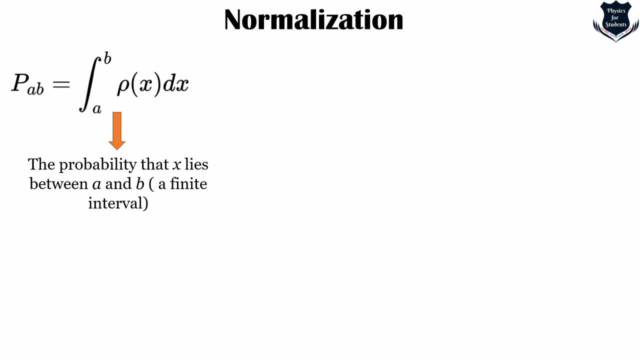 So this is the proportionality factor. rho x is often loosely called the probability of getting an electron, But it is a very sloppy language. It is better to Use the term probability density. So the probability that x lies between a and b, which is a finite interval, is given by this integral sign, followed by a, rho x and the differential value. 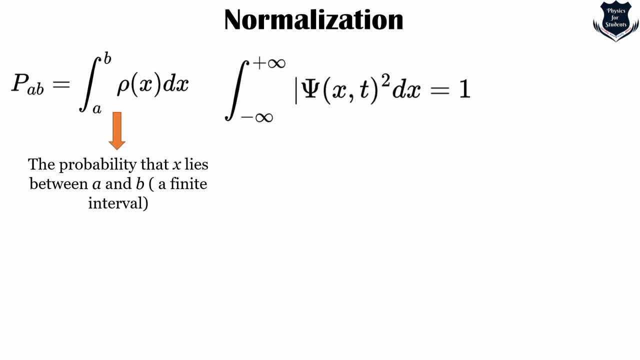 Okay, So we now return to the statistical interpretation of the wave function, Now you see, which says that if I psi x, comma t squared, is a probability density for finding the particle at point x at time t. So it follows from this equation That this one must be that the particle got to be somewhere else. 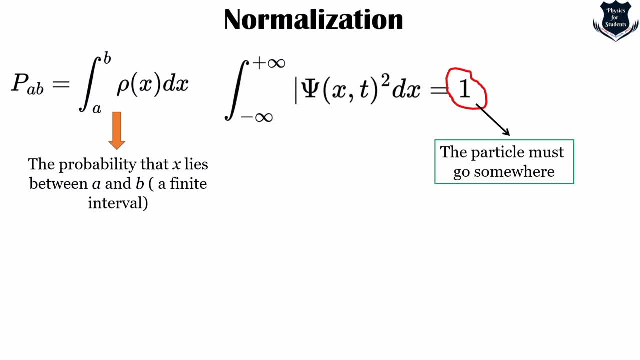 Right. So we get a value, for example van 1 out of this wave function, And it says that the particle must be somewhere. Okay, So now the problem is that, after all, the wave function is supposed to be determined by the Schrodinger equation. 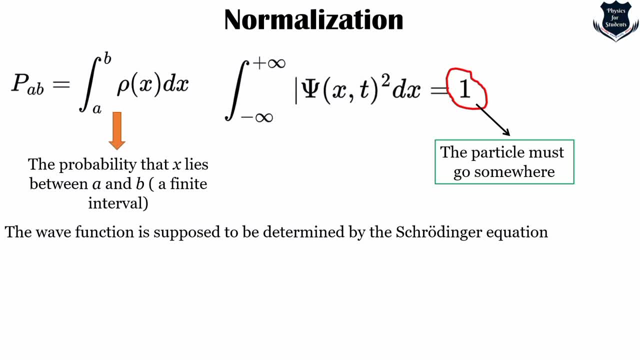 Right Now we cannot impose- I mean to just put- an extraneous condition on psi, its psi Greek symbol, without checking that the two are equal. If you look into the equation, this one, so I would put two Schrodinger's equation. 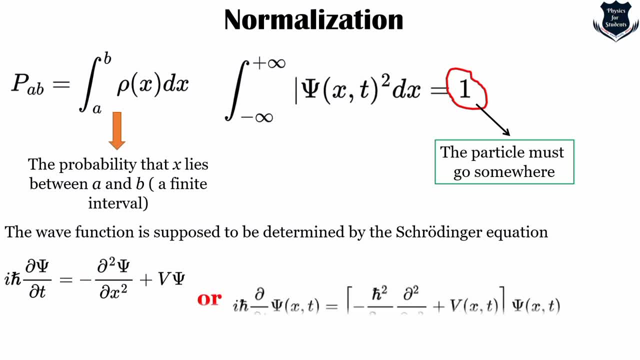 I mean to say two ways of putting Schrodinger equation, One is this one and one is this one, So both of them are more or less the same. So this part, that is, psi x, t, is a solution Right, Because the wave function is determined by the Schrodinger equation. 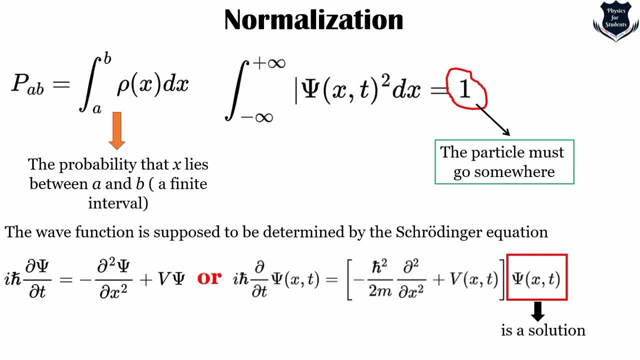 So this has to be a solution. Considering this: psi x t. If I take another one, say psi x t, Where a is basically a kind of a. you can say an, any kind of a complex constant. So why I am stating this? 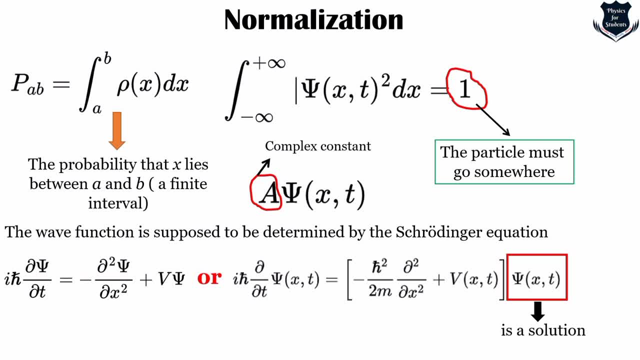 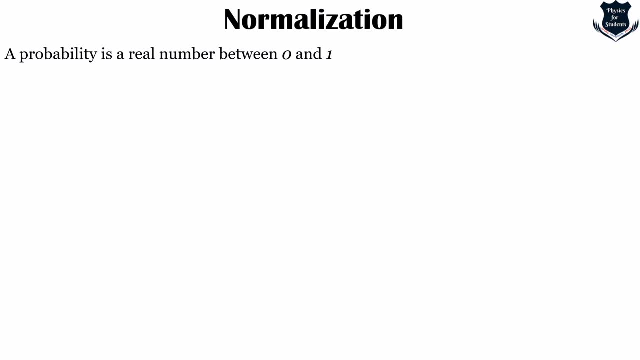 Because we must do that is, pick this in the undetermined multiplicative factor So as to ensure that this equation is satisfied. So, in order to do this- that is why we call is a normalization. Okay, So the probability is of a real number which lies between 0 and 1.. 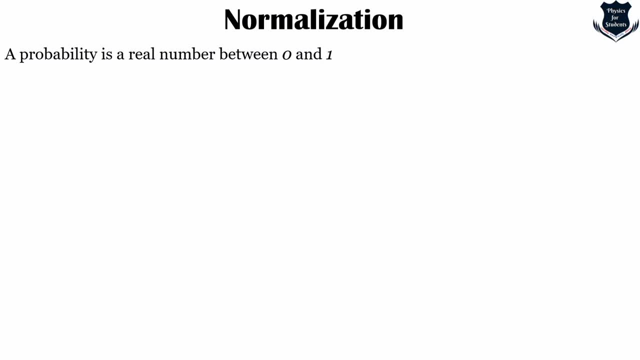 So what does it Mean? is that an outcome of a measurement which has a probability 0 is an impossible outcome, And when an outcome which has got a probability 1 is a certain outcome, right. So these are the two values. Now the probability of measurement of x: right. 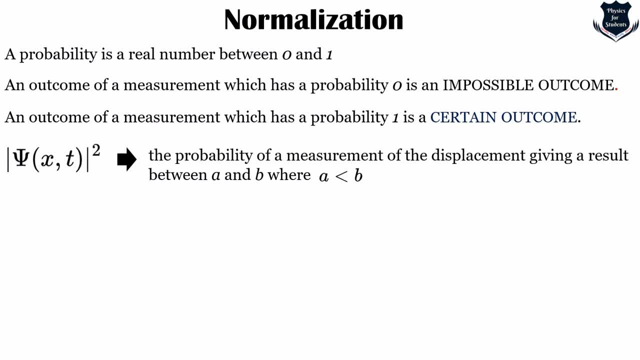 Which yields to this value is something which is given by the displacement that a is less than b, And if I use the little bit of a set theory kind of a, this is easier. So p sub x, which is In which belongs to a comma, p of t will be the integral of a to b, squared by its probability density, followed by dx. 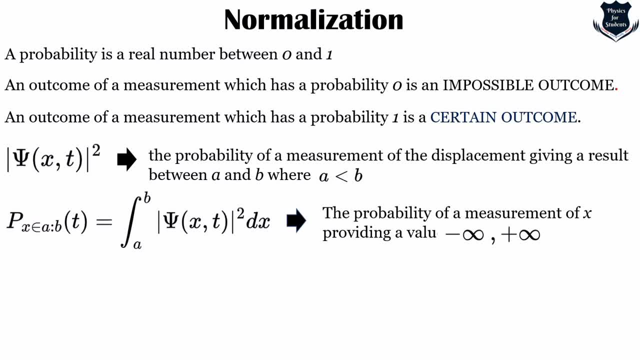 That means the probability of a measurement of x is between the providing a value between minus infinity to plus infinity. Further, if we take this one, which is basically the, again we can take this one. This actually measurement of x must generate a value between minus infinity. 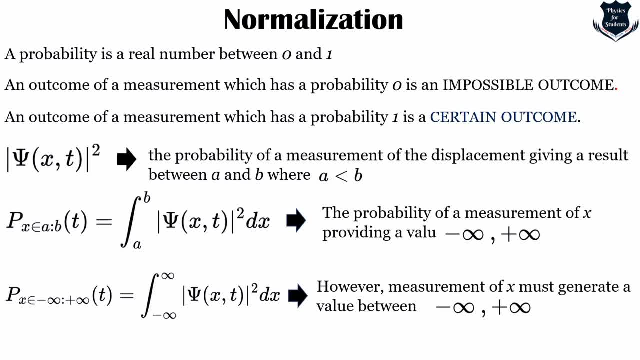 To plus infinity. So this actually shows that how the measurement of the value which ranges between minus infinity and plus infinity should be. So first is that 0 is an impossible outcome. We need to find somehow Now we will look forward that- how we can get the normalization value to 1.. 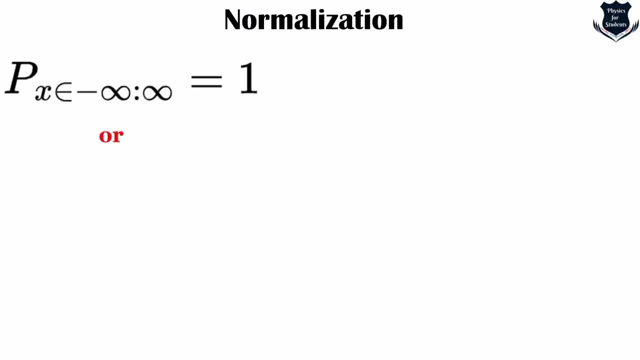 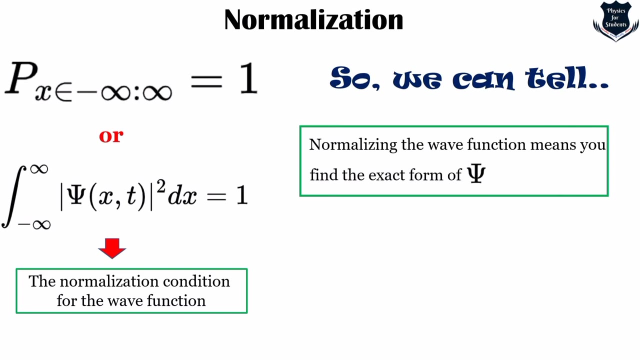 Okay, so it should be. this equals to: we can use the set theory notation or we can use this. Both of them are the same. So this is the normalization condition of the wave function, And from here what we can tell is that normalizing the wave function means actually to find out the exact form of site. right? 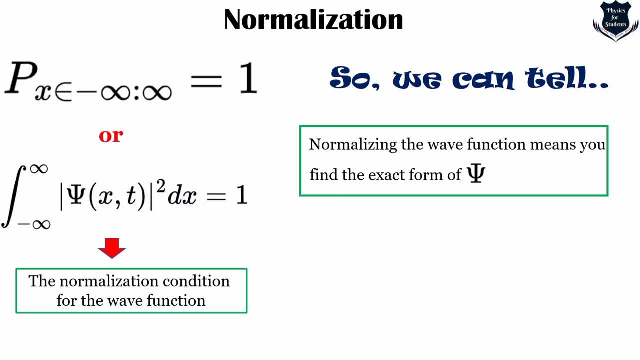 So until we find the exact form of side, you understand, we cannot find the basic value of the electron. So it is quite clear till now that the need for the normalization is to locate or find the exact form of a wave equation. Until we find the exact form of wave equation or a probability, we will be unable to do the mathematics. 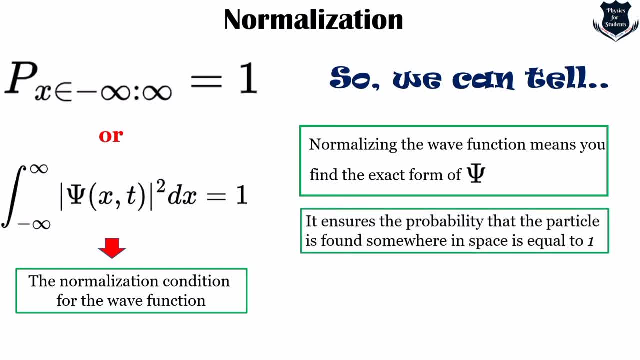 So it ensures that the probability- the probability of the particle is somewhere spawned between equal space- is equal to 1.. So what happens is that the normalizing, the wave function gives them a coefficient, such that the coefficient squared is the probability. That means this x comma, t squared is the probability of finding the particle, etc. in that eigen state. 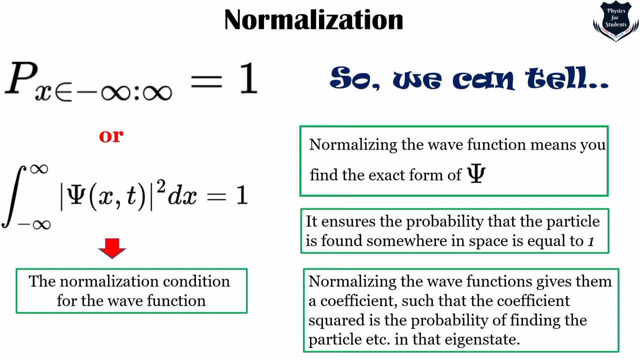 Now, don't worry, if you don't understand what is an eigen state or an eigen value, I will soon make another video on eigen state where I would be explaining this. But just understand that it is a state where there is a probability of finding the value. 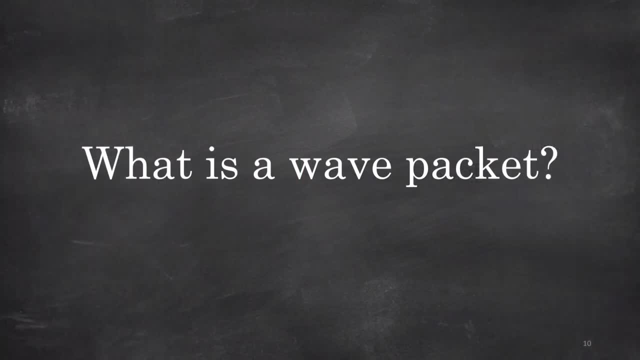 Okay, Now, before we move ahead, this is the. this is what is called normalization. Now we need to show this normalization through some examples. Now, before I go ahead and explain you the example, the first thing I need to tell you a little bit is what is called a wave function. 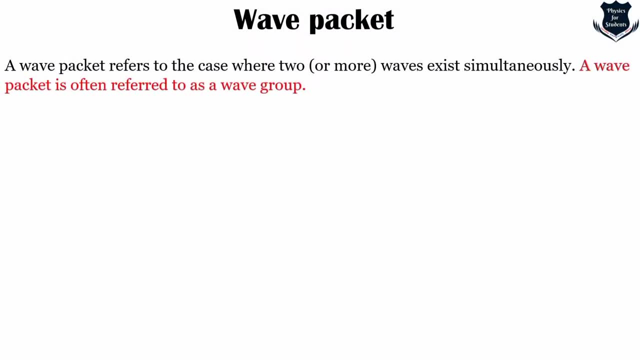 Now a wave packet is actually refers to the case where there are two or more simultaneous waves that exist, and a wave packet is often referred to as a wave group. Now the situation is permitted by the principle, what is called superposition. This principle states that if any two waves are a solution to the wave equation, then the sum of the waves is also a solution, and it holds in case of a linear system. 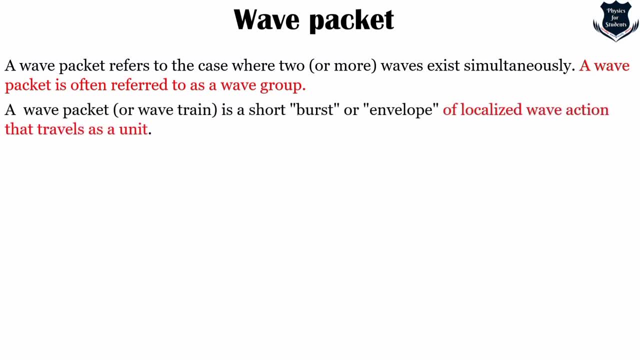 Now let me show you a demonstration. So a wave packet or a wave train also, is a short burst or envelop of a localized wave action that travels as a unit. Now let me show you this is a say, for example. it is a kind of a waveform. 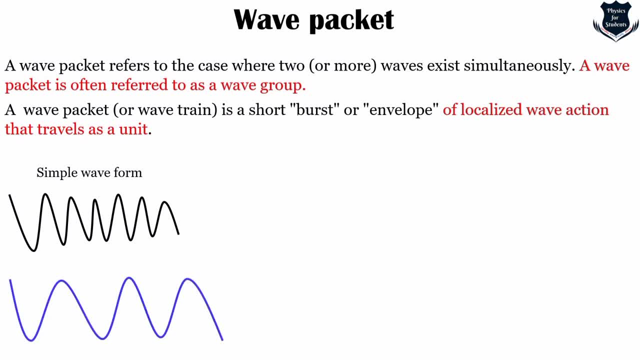 So I take it as a simple waveform, the black one, Then the blue one, for example. it is some kind of a wave, but it has got a different wavelength Right, As you can see from the. you know, the horizontal distance between the two crests and two troughs are different. 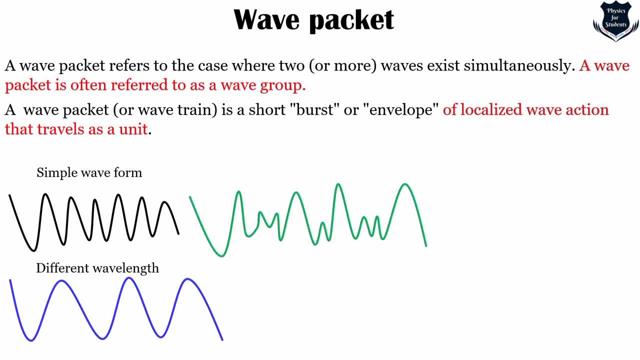 Right Now, the wavelength of this one- this green one, is basically what I call- is the sum. It is the sum of the two waves, Right? So this is called the sum of the waves, or packets, Right? So this green curve shows that it is the sum of two waves. 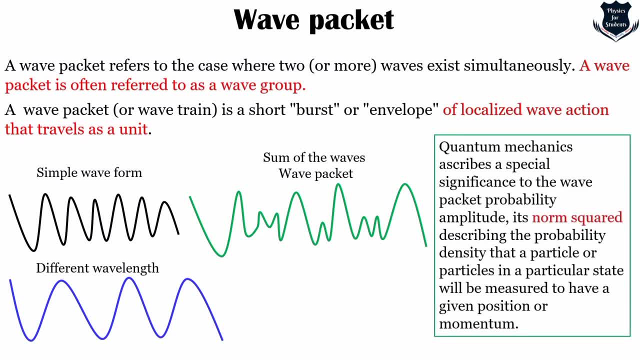 Now what happens? Quantum mechanics actually provides a special significance to the wave packet. It is interpreted as what is called a probability amplitude And its norm is norm. That is, the vertical part is squared- describing the probability density that a particle or particles in a particular state will be measured to have given a position or a momentum. 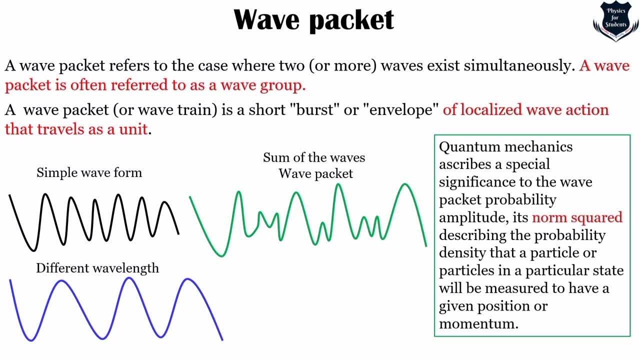 These are the two factors which has been later described by Heisenberg's Uncertainty principle. Without that we cannot locate it Right. So clear till now. I hope it is going quite well. So the probability that a particle or particles in a particular state will be measured, given a position or momentum, 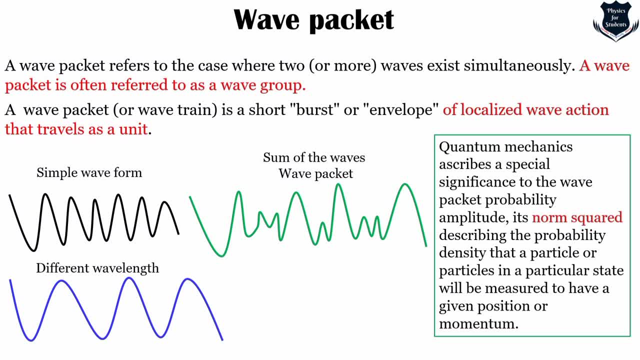 Now the wave equation. in the case of a Schrodinger wave equation, And through its application, it is possible to deduce the time evolution of a quantum mechanical system similar to the process of a Hamiltonian, which we know is a formalism of classical mechanics. 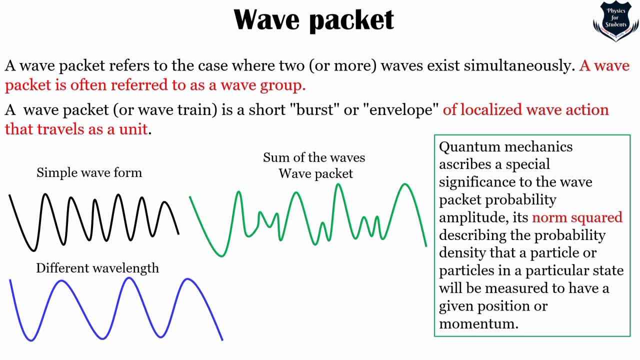 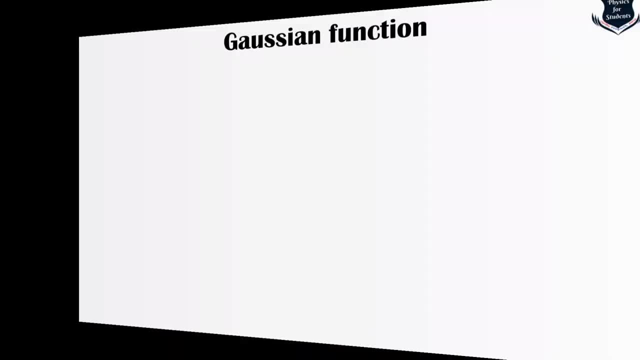 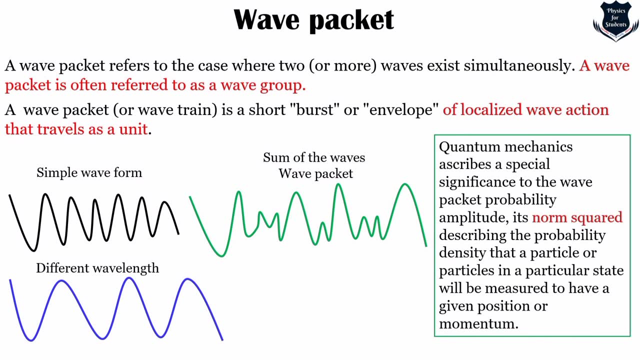 The dispersive character of solutions of Schrodinger equation has played an important role in projecting Schrodinger's original interpretation and it has been accepted by the Ward rule. So that is a different issue. So now you understand from this part that we need what is called. what is called is a wave packet. 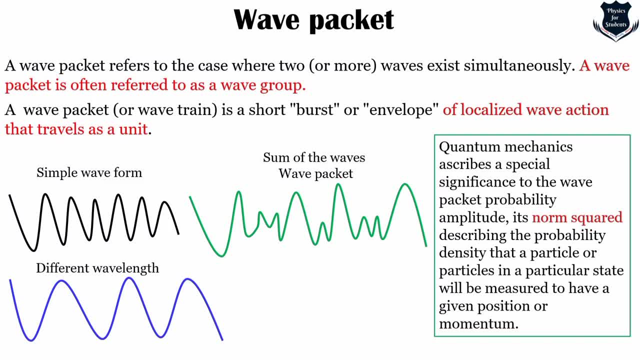 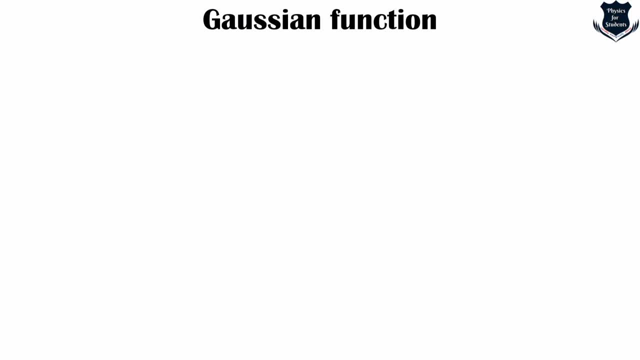 Because it is a sum of the waves and quantum mechanics gives that value which is to be squared. Now I will quickly explain you, although you might be knowing that, what is called a Gaussian function, Gauss's function. If I get a kind of a bell shaped like this and I draw a vertical line, 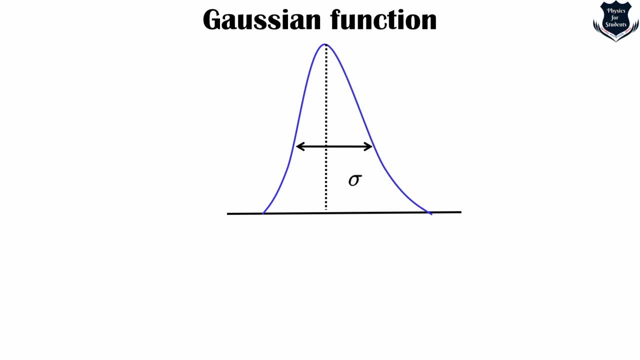 So this is the sigma which tells the bit. So this is what is equal to the wave function and it equals to the Gaussian function. This is called the Gaussian, And if, in case that the sigma Is equal to infinity, the Gaussian is infinitely wide, right. 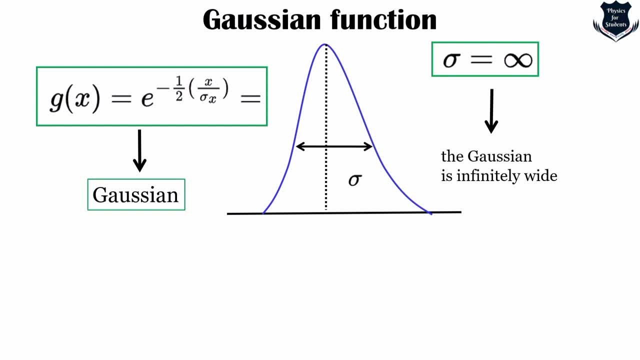 So what does that mean? It means that to construct a constant, one only needs the infinite wavelength. to construct something narrower, narrower than a constant One, needs more and more wave numbers. So to construct a very sharp Gaussian, you know where X is tending towards 0, right? 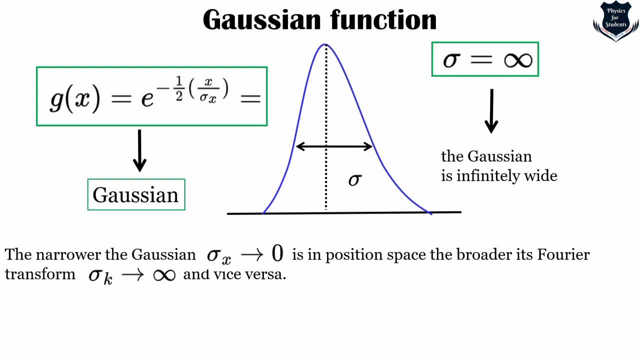 The Fourier transform actually flattens it out, and one needs an infinite wavelength. So we need an infinite number of wave, number waves to get an infinitely sharp features. obviously, As you know, if we shift the Gaussian, then the Fourier transform rotates by a kind of a phase. 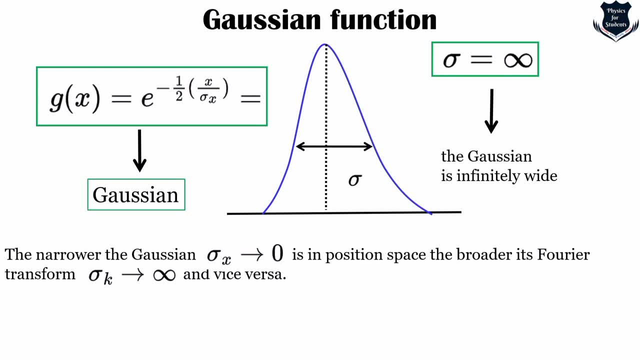 And, conversely, if we shift the Fourier transform, the function rotates by a phase. But fortunately, even with the extra phases, the Fourier transform of a Gaussian is still a Gaussian, So we will use this Gauss's function or the Gaussian function in order to get this. 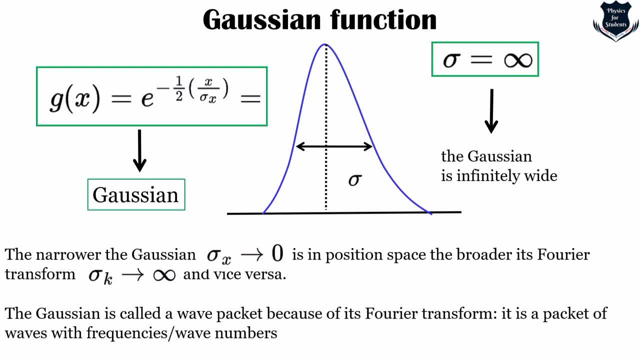 The Gaussian is called a wave packet because of its Fourier transform. It's a packet of waves with frequencies and numbers. So that is how, why I told you that we need what is called a know what is called a wave packet, And this is how the wave packet is related to a Gaussian function. 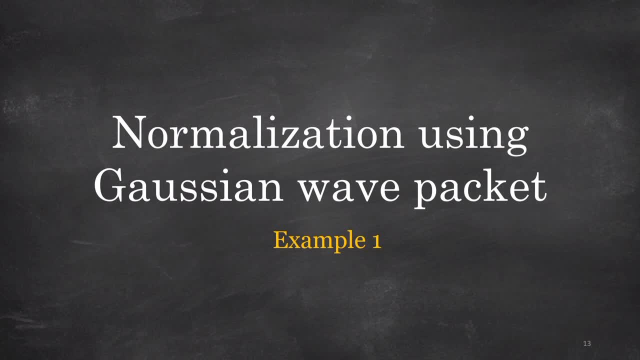 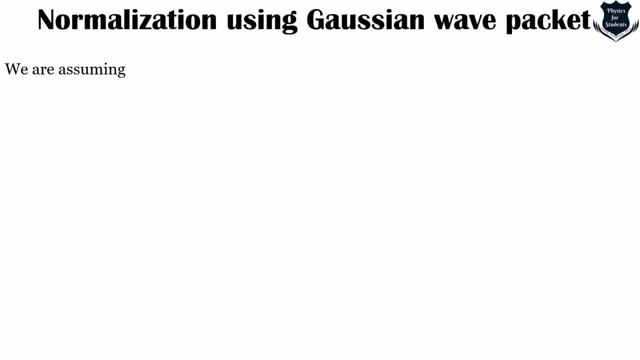 And it is called a Gaussian wave packet. Okay, So coming up now is the first example of normalizing using a Gaussian wave packet. So we are assuming, in case, that X is equals to X0 and this yields to this one. 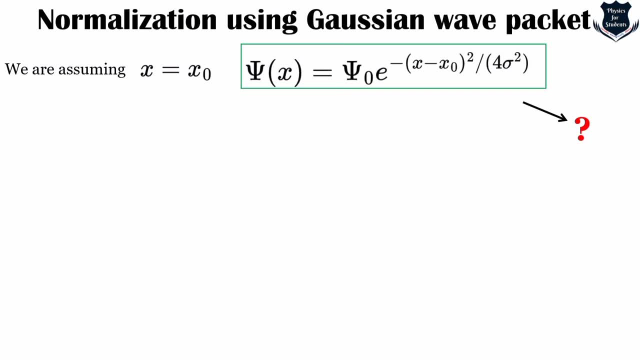 Now, don't worry if you really don't understand this, because this is some kind of a time evolution of Gauss's law, which I will put up, surely, in the next part of the video. But let us assume this Now: in order to determine the normalization constant, that is, psi sub zero, 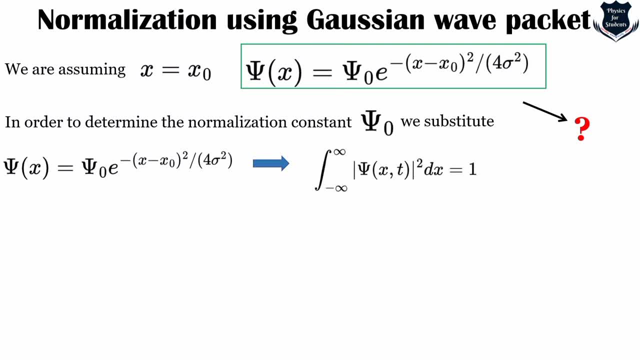 we substitute this value into this one and we get this one Right. So we are substituting this value into this equation And we are getting this one. If we change the integration, Y equals to X minus X0, followed by this, then what we get is this one. 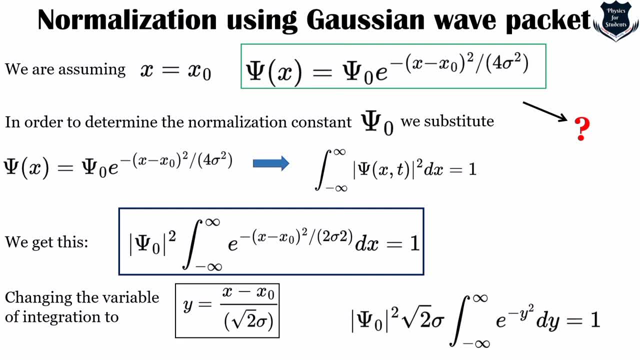 And you see, already we are getting a one, Isn't it? So we just substituted each one of these values and change the integration value, And what we get is this one. Okay, So we move on to the next. So we already know that this is this. 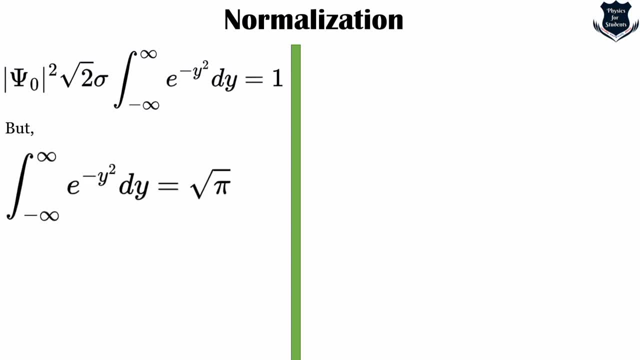 Right, It is this one, And from here we know that this is pi. This is just pure mathematics. You can look into this which yields to this, And we get this one, And this is actually what is called a generalized normalized, general normalized. 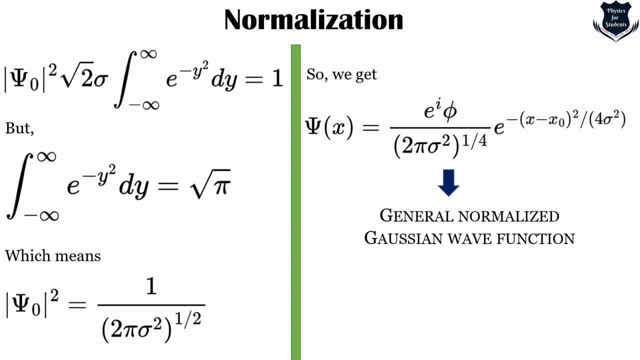 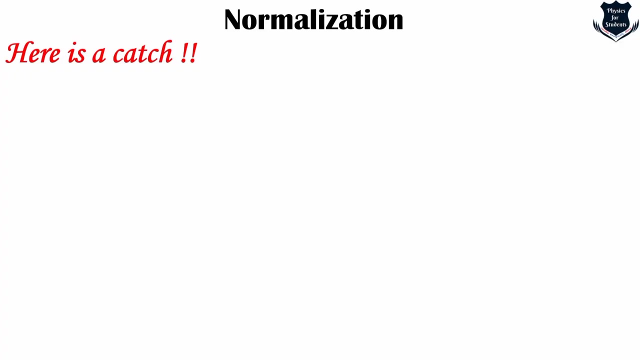 Gaussian wave function Right. So this one, this value, is basically what is called an arbitrarily real phase angle. So this is an example which shows, I mean to say, how we transform a general, normalized Gaussian wave function. We will use a quick and a very simple formula example using Schrodinger equation. 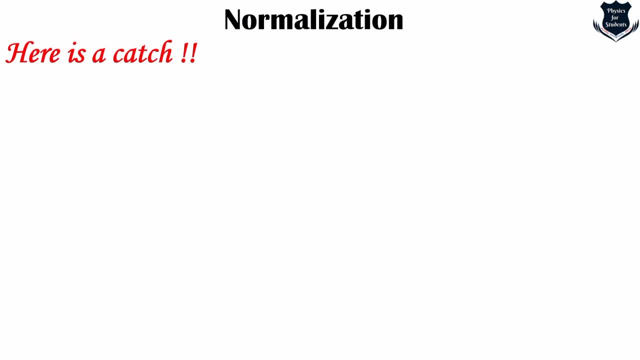 Now remember that when we are doing a Schrodinger equation, there is a small catch. The catch is that if we have a normalized wave function that is already, you know, a kind of a t equals to zero, then how will I know that it will stay as normalized as psi grows? 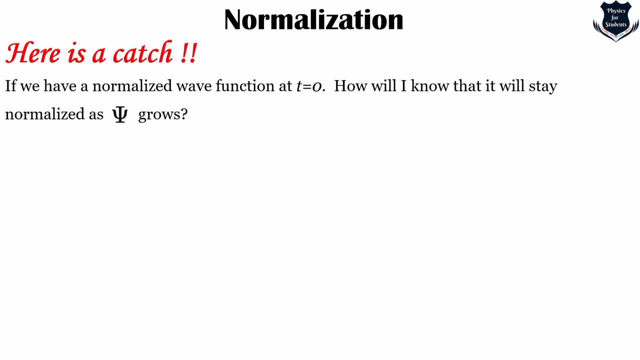 That means that with the passage of time, which is called a time independent Schrodinger equation, how will I know that it grows? So if a wave function is initially normalized, then it stays normalized as it evolves. If this is not the case, then the probability interpretation really doesn't make any sense. 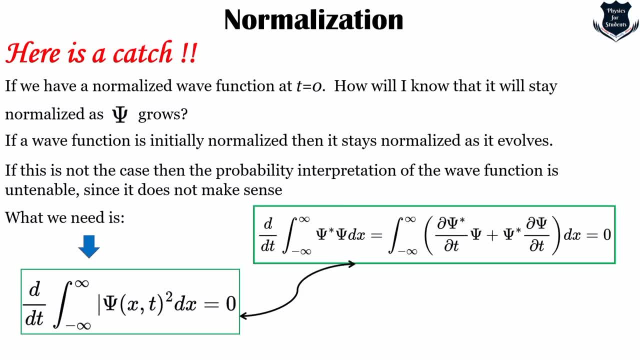 So what we need is this one, where value will be equal to zero, And this is something which we put it up in the Schrodinger equation. So sorry, let me show you once more. So it actually satisfies this one through this equation: 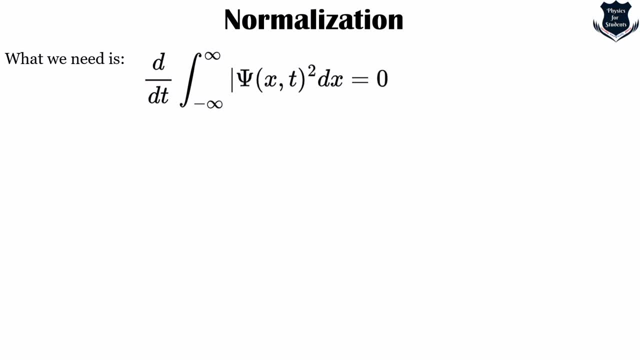 So we will just take the same equation. What we need is this: Now, if I take a complex conjugate of this one, I know it is very weird, quite long equation, but you can just check out those calculations later and you can let me know how it happened. 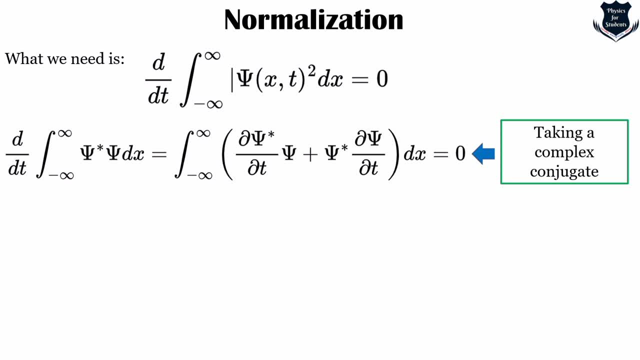 in the comment section. So we are taking the complex conjugate of this which leads to this, And if I multiply the Schrodinger equation with this one, that's the complex conjugate upon i h bar, then we get this one right. 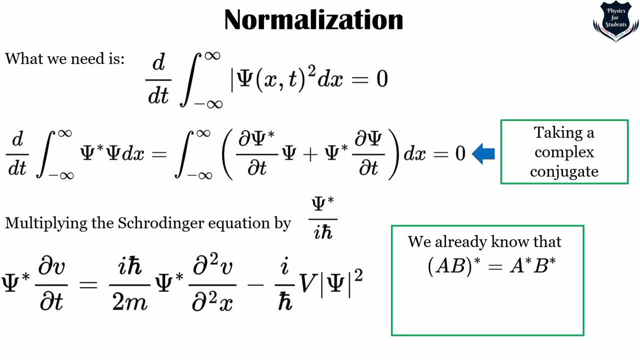 And we already know from the formula of complex conjugate that a, b conjugate is equal to a conjugate, b conjugate And if you take a double conjugate, obviously it will give back to the original a and the conjugate of i is minus i. 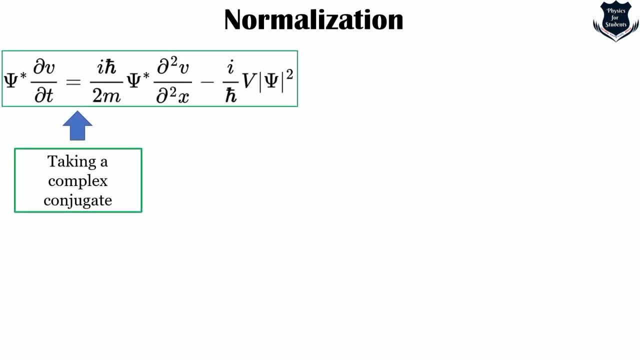 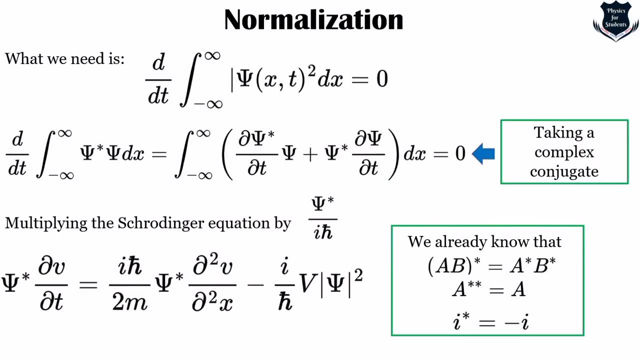 Because we know this, then what we do is that we take a further complex conjugate of this, which leads to this: You can go back to the screen and just take a snapshot of this page, right? So we already know this from here. 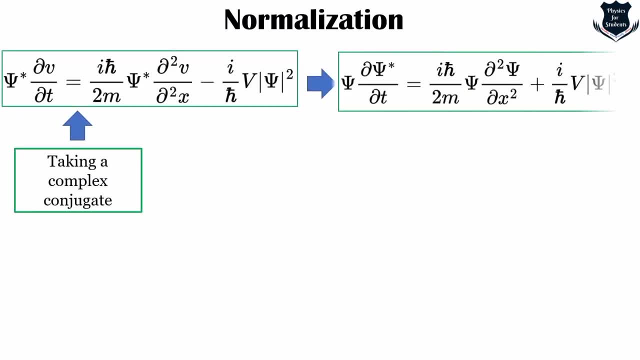 We come to this one and we are taking a complex conjugate. So you see that complex conjugate of the first wedge function psi star removes, and then it goes into this and this middle psi star removes in this simple way. So we can combine these two equations further back into this one right. 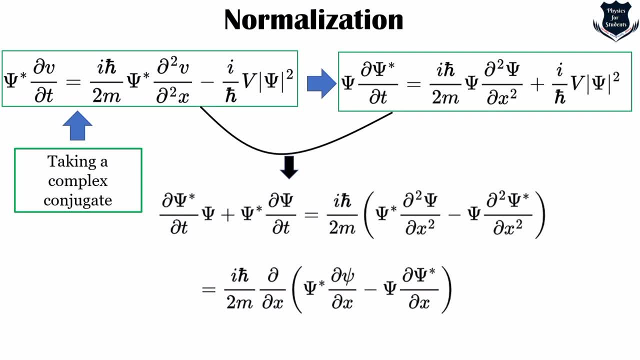 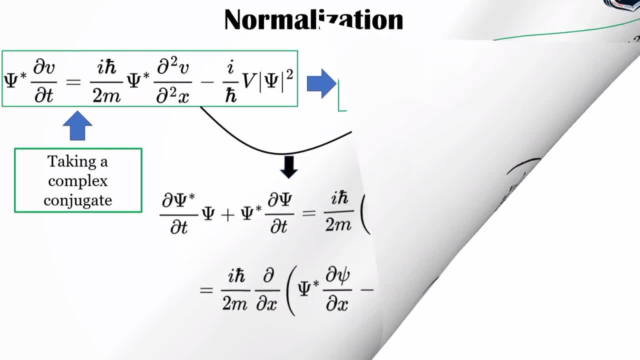 So we just combine these two equations and we got into this one. You can take a kind of a snapshot, if you want, or any other further details that you want to take a note of this screen you can. So now what we do is that we are okay, so we got these equations right. 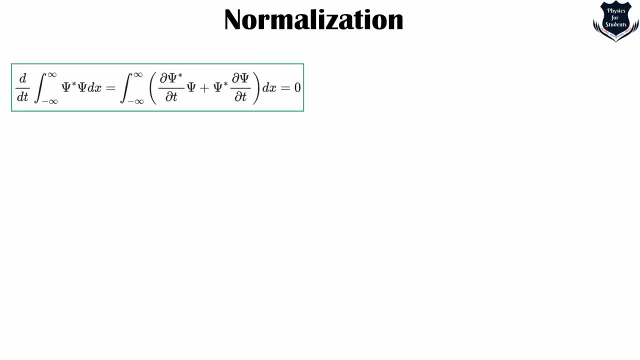 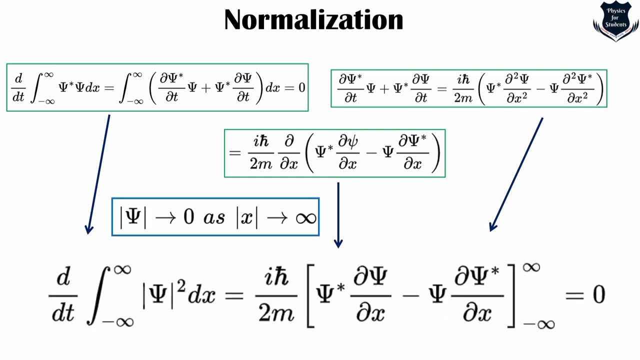 One, two and this one big one. So now what we will do? we will sum up this equation: this one, this one and this one taken together, What we get is this right, And this is true when this moves to zero as x moves towards infinity. 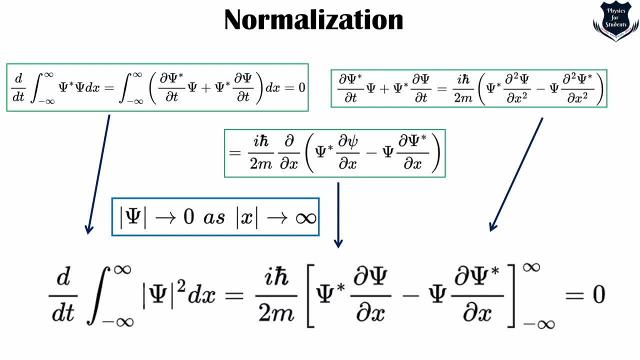 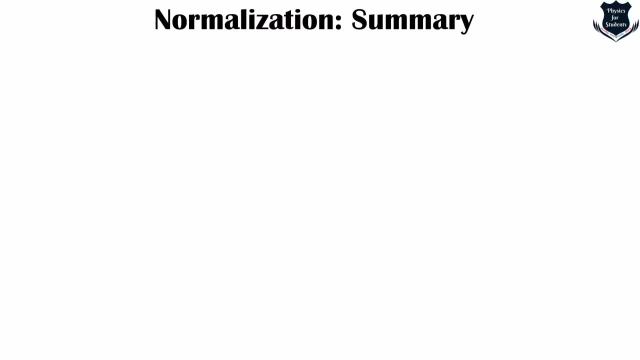 So this is again the normalization using the Schrodinger equation. We wanted a zero, which if you go back to the screens and you will see, and we have e to zero. So what can we summarize? Can we summarize? what do we mean by all those normalization methods? 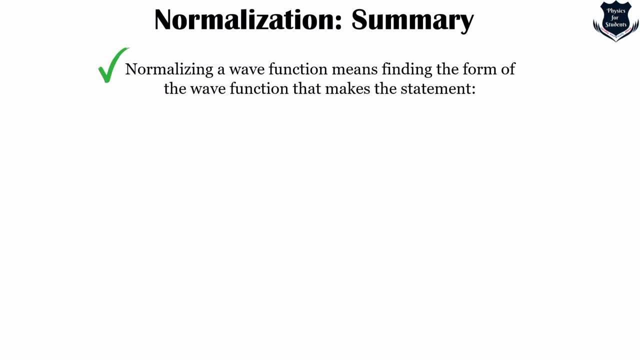 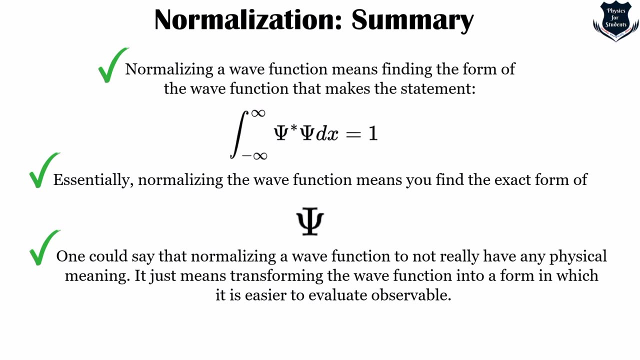 So normalizing a wave function means finding the form of the statement, this one which we have already seen. the value should be one. Essentially, normalizing the wave function means you find the exact form of the wave function, psi. One could say that normalizing a wave function to not really having any physical meaning until and unless. 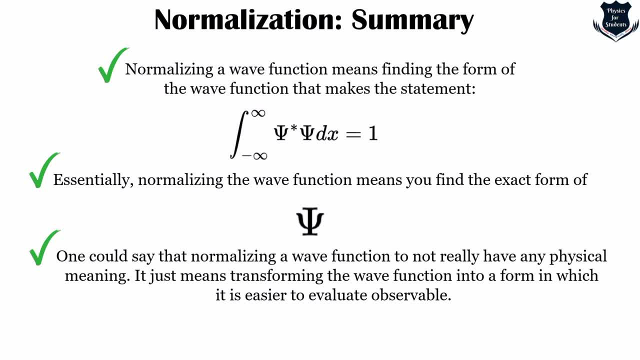 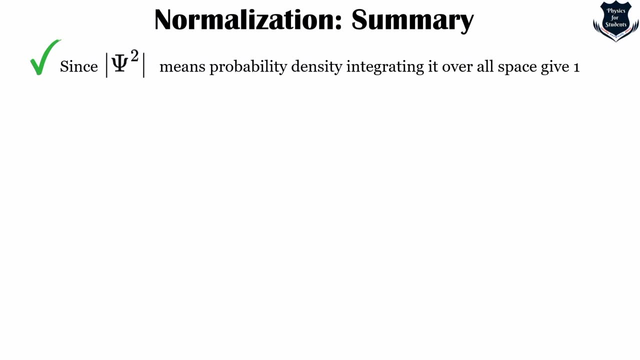 where the wave function takes the form so that it can be easily evaluated and observed. Obviously, it really doesn't have any significance until we evaluate and find out an observable, And that is the reason for a normalization. Further, I would say that since psi square means the probability, density, integrating it all over space, it gives one, which means we are. 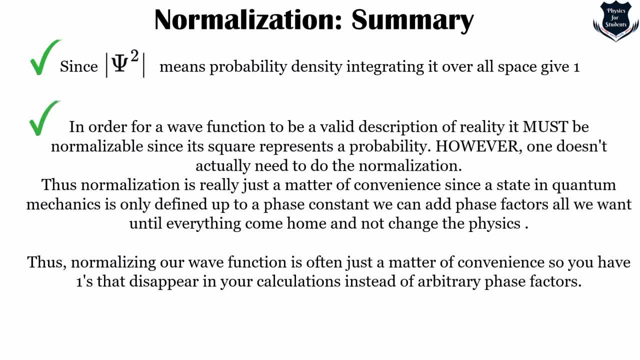 it is not probable to find out. hello, Here is a better and a clear description. In order for a wave function to be valid description of reality, it must be normalized. Why? Because one does not. actually. it squared represents the probability. Thus, normalization is really just a matter of convenience. 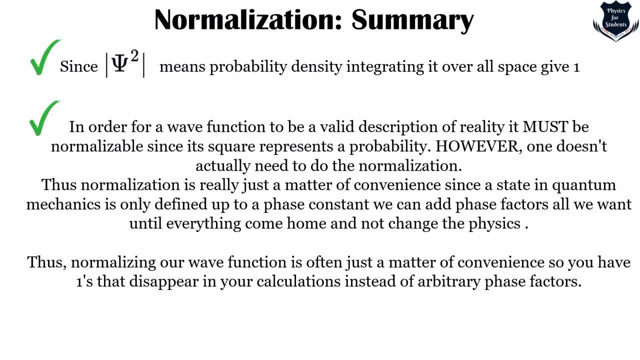 Since the state in quantum mechanics is only defined up to a phase constant, that we can add phase factors and all we want until everything come home And physics really do not change. That's true because we really don't want to change things. So we need to normalize and get a kind of a predictable value. 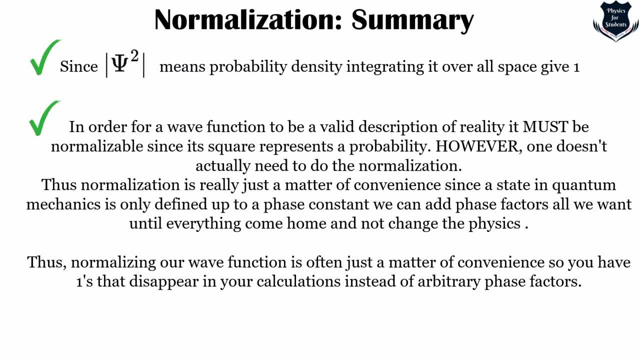 Thus normalizing our wave function is often just a matter of convenience, So you have ones that disappear in your calculation. instead of arbitrary phase factors, This is a more kind of a clear literal description, A layman's understanding that it must be normalized since it represents. 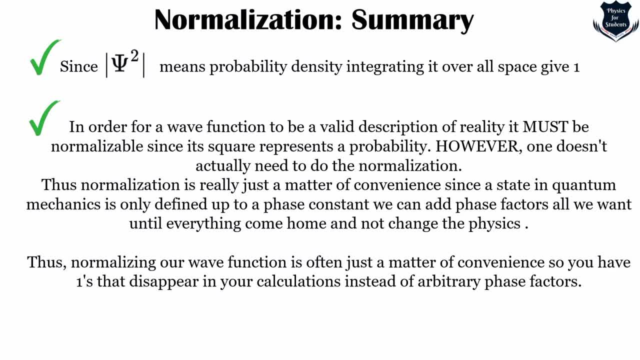 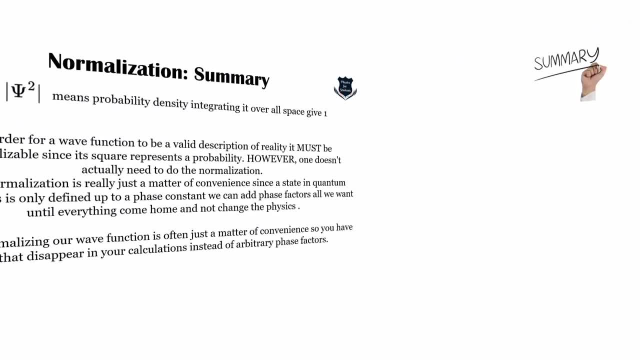 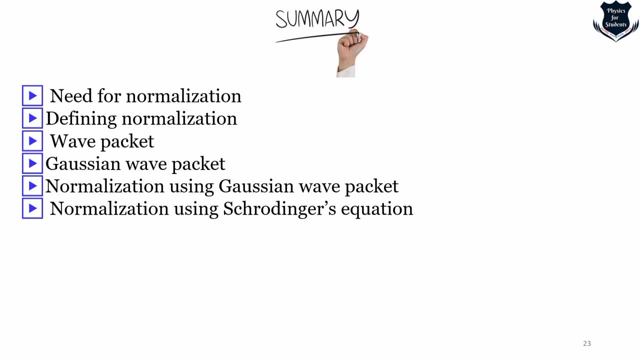 square represents a probability. However, one does not actually need to do the normalization. It is required so that all things come home and everything doesn't change and leads to bad physics. So what do we summarize? We summarize: we have understood the need for a normalization, defining a normalization. 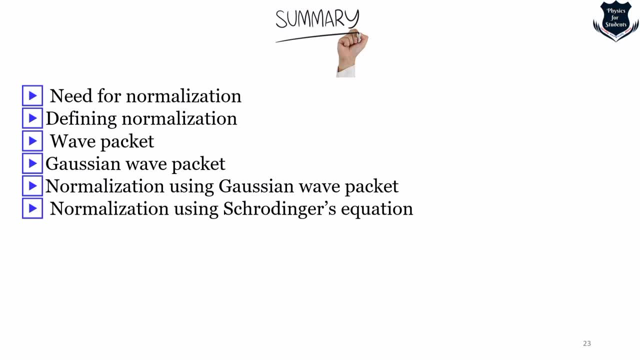 We have also got a hold of what is a wave packet, Gaussian wave packet, normalizing using Gaussian wave packet and Schrodinger's equation. So in my next video, what I would be doing is that I would be speaking a bit about 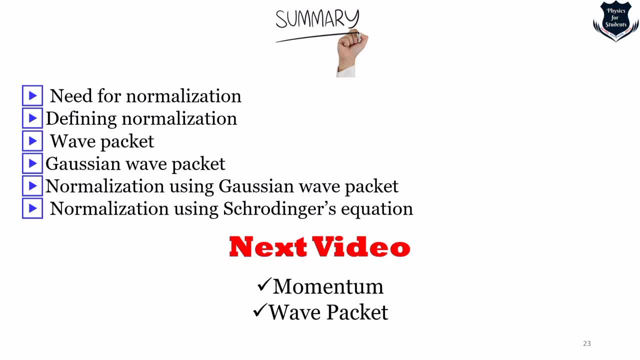 what is the momentum in quantum mechanics compared to that of classical mechanics and what is a wave packet right? So that's all for today's video. I hope you liked it. I'm making the quantum mechanics videos a little bit shorter in length because I think that each video, if it is dedicated to each concept, 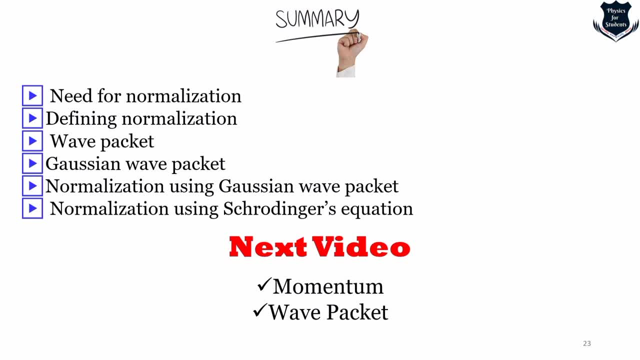 that is much more clearer, elaborated and understanding is much deeper. Thank you for watching this video on my channel. Please do subscribe, like and put up your comment in the comment section, And click on the bell icon to get all the notification from Physics for Students.